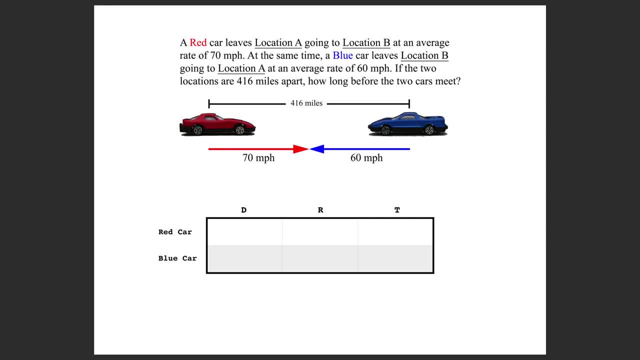 Next, let's fill in what we know. We know the speeds or the rates for both cars. Now we must declare or assign a variable we're trying to find. Most math teachers want you to do so In this case. let t be the length of time for two cars to meet and fill in the variable t. 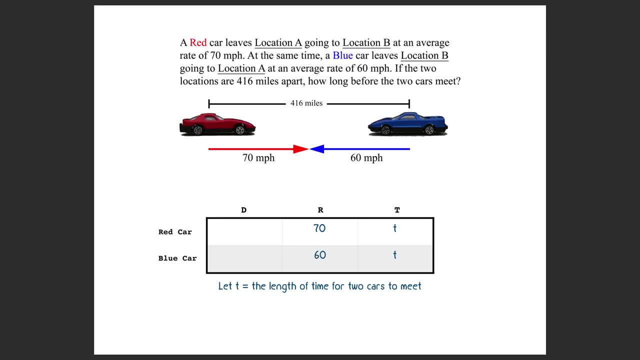 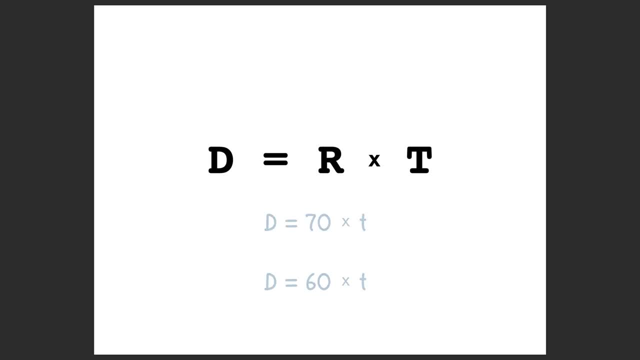 t is exactly what we're looking for. Both cars take the same amount of time before they meet. Well, here's what we need to use: Distance equals rate, times time and, with direct substitution, 70 times t for the red car and 60 times t for the blue car, Give us the two distances we can fill in. 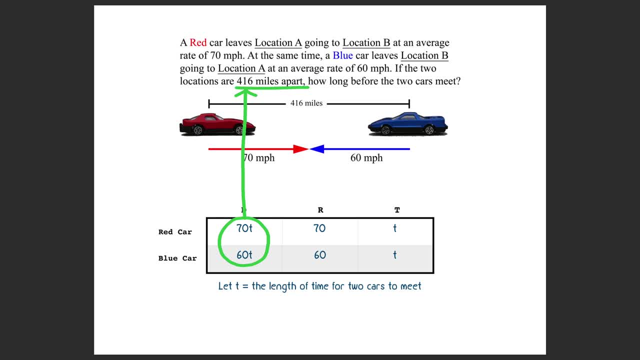 the table, Since they travel certain distances before they meet, being 416 miles apart. try to imagine painting the tires with never-dry, never-run-out-of-paint red and blue. They would paint the road with certain distances Before they meet. the red car would paint longer distance than the blue car. 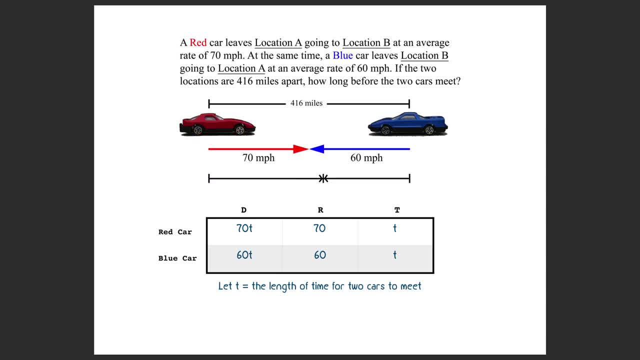 because it travels faster. So we have two distances in the table: 70 times t for the red car and 70 times t for the blue car. So we have two distances in the table: 70 times t for the red car and 70 times t for the blue car. 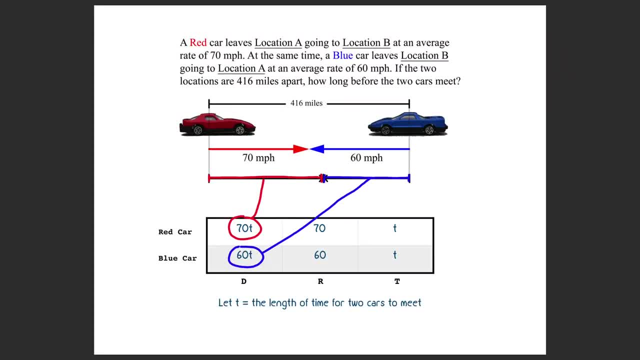 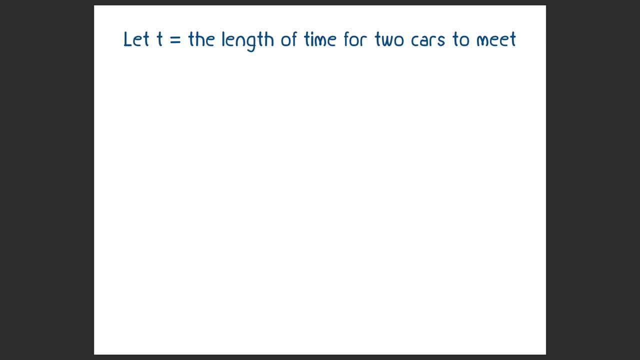 70 times t represents the distance for the red car, 60 times t for the blue car, and we know they must travel a total of 416 miles before they meet. We can now set up an equation: 70 times t plus 60 times t equals 416.. Combine like terms: 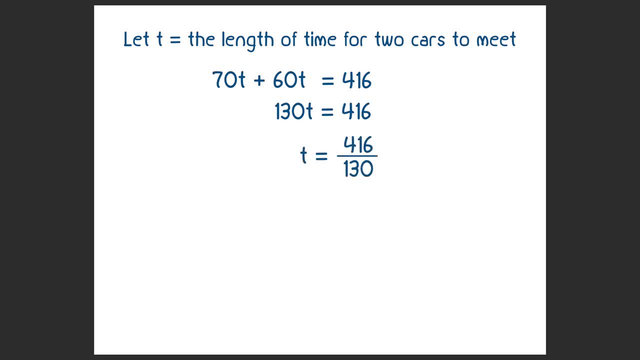 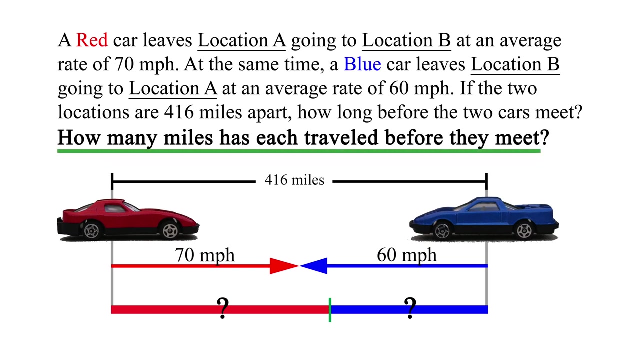 130 times t equals 416.. Divide both sides by 130 and reduce or convert into a mixture. Now we must think about a numerical argument. If t equals 416 and g equals it equals 1, then if t equals 3 and 1. fifth, 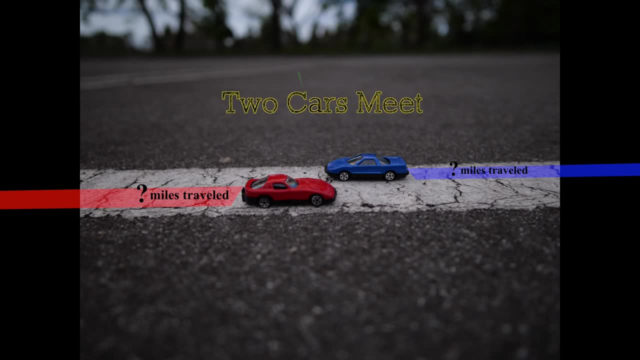 then this윾t equals 3 and 1 fifth hours. It's 3 and 1 fifth hours and it equals 4.. Referring back to the table, we know the distance for the red car is 70t and the blue 60t.